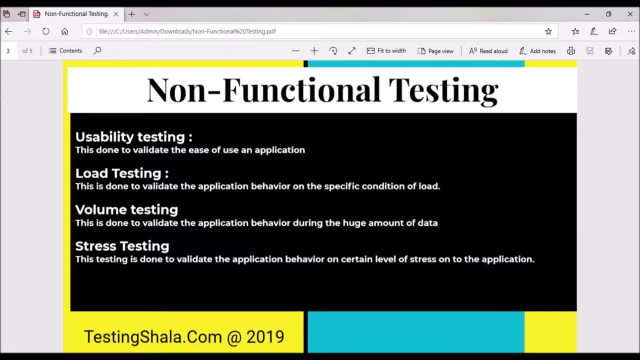 also watching how much the memory is going to consume. so the third: volume testing. so volume testing: here we will be validating the application behavior by putting the huge amount of data. let's say, if you instruct, import thousand users, two thousand users, one lakh users, million users, then we will see how the application is going to behave during that time. so that is the kind. 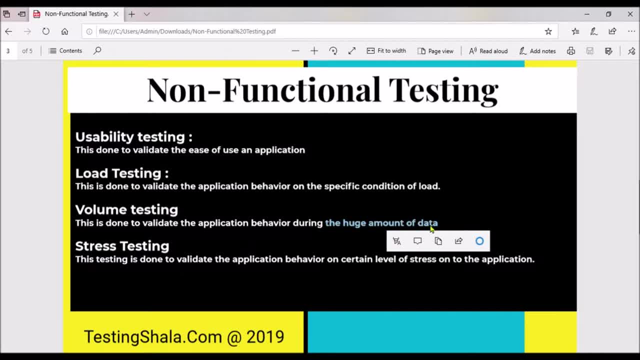 of testing. we call it as a volume testing. the fourth type of testing is stress testing. here we will be continuously going to stress the application by, let's say, one million records, two million records, ten million records, and we'll be keep watching at what stage this application is going to crash. 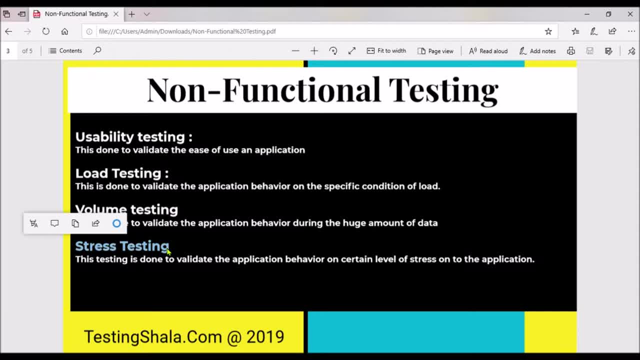 our application is going to behave in a totally different manner, so that is called as a stress testing. basically, we are going to stress the application in a different interval by putting the appropriate load to the application. hope you understood the four different types of testing: usability, load volume. 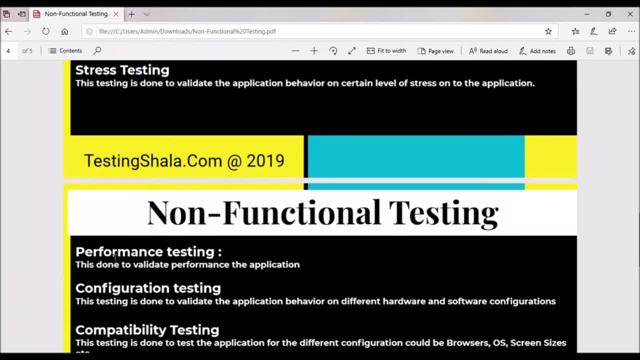 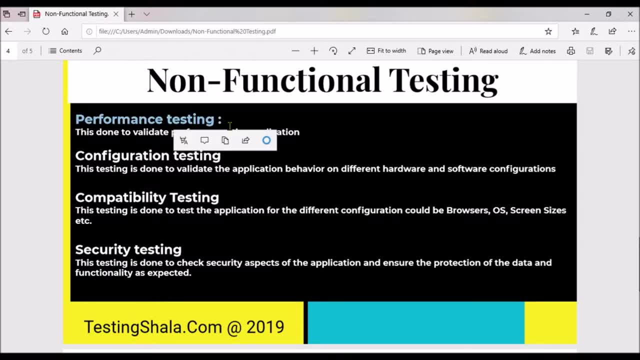 and stress. then let's move on to the understand. remaining another four non-functional testing types: the performance testing. the performance testing is done to the application to validate all the response time and various other factors under the performance will be validating under this type of testing. then let's move on to the 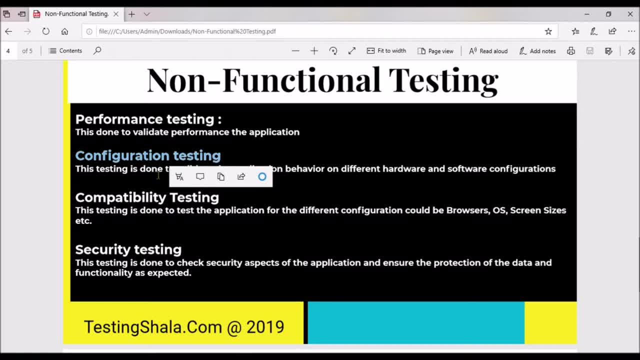 testing. six type of testing is configuration testing. this is a kind of testing. we will be validating the application behavior with the different configuration of hardware and software. let's say, if the applications are going to be deployed on android or ios or windows, in terms of mobility, in the same way, if you are going to deploy the application in red hot, linux or solar is. 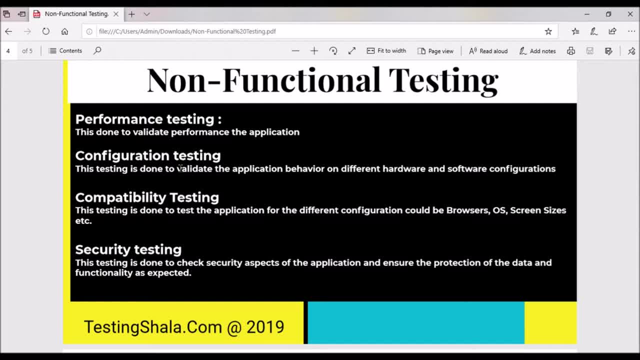 windows, how the application is going to behave in a different manner. that is the thing we are going to test it. in configuration testing. we will also be validating in terms of what kind of databases- what i call sql, what environment this vertical sql are going to rely on and with 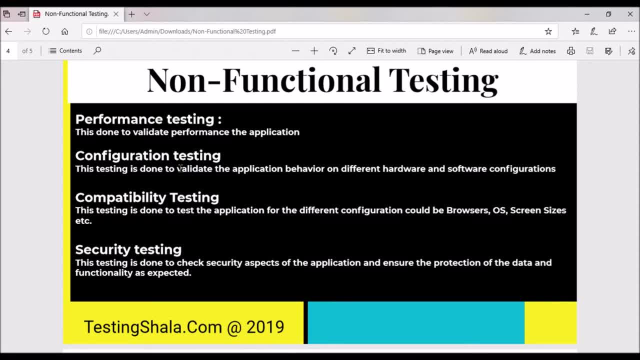 all these different conditions, including the application server, web server, with the different hardware and software configurations. we'll be testing it as part of a configuration test. the seventh type of testing, which is compatibility testing: this is done to by putting a different configurations, such as browsers ois screen sizes, just to validate whether the really the application. 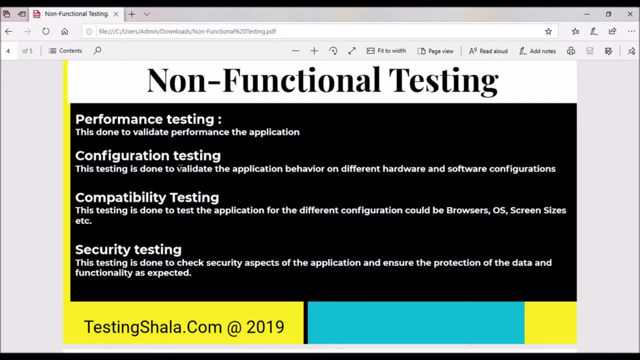 still behaves as expected. sometime we will also validate at fixing the issues to the previous releases just to see still the applications works in the previous releases and so on. as well as the printer pieces means new releases, so that is a kind of testing. is called as a 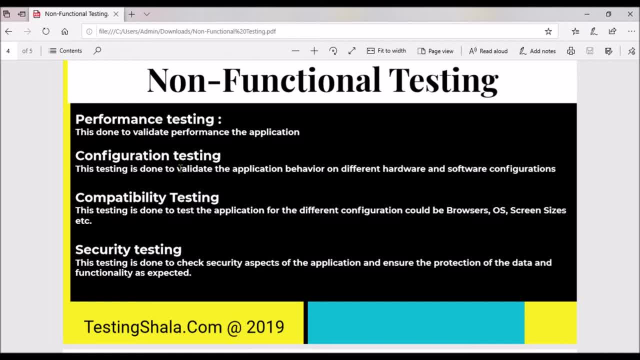 compatibility testing. the last type of testing under non-functional testing here is security testing. security testing is one of the important testing which we do to ensure there is no breach in the security aspect of the application. basically, here we are going to ensure that the client data is secure, to protect the client data or personal data from the application. 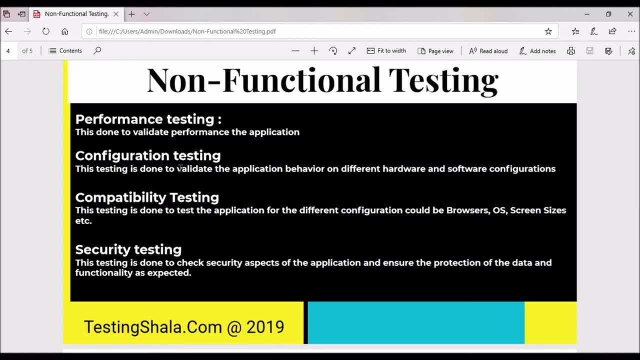 from the external people who are unauthorized people to access the application and act the application to access this important critical data. we have to ensure that those things should not happen. so this is a testing where we are going to adopt security testing to ensure we is no compromise on the confidential information. i hope you understood all the different a types. 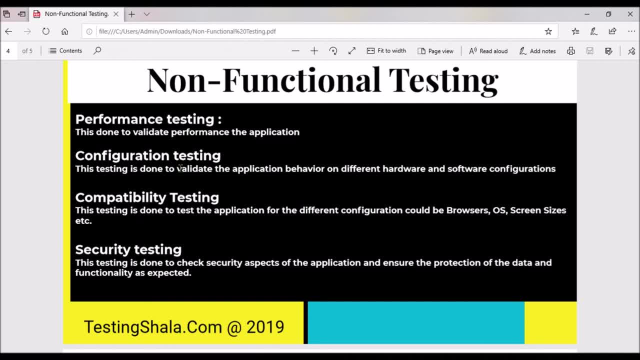 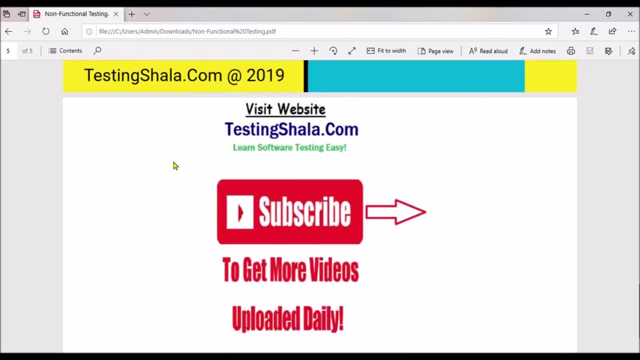 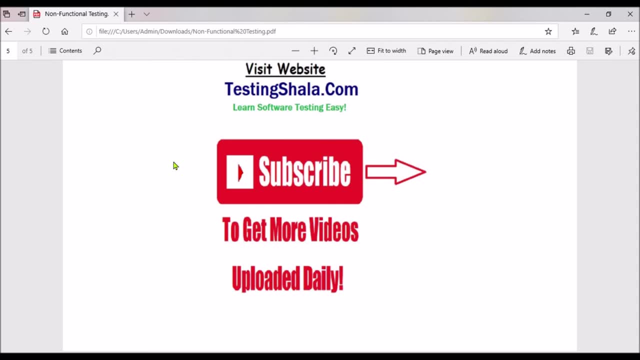 of testing under non-functional testing category. if you like this video, please click on like button if you are visiting first time to the testing shala, testing shala is focuses on learning software testing very easily and if you would like to get similar kind of videos related to software.